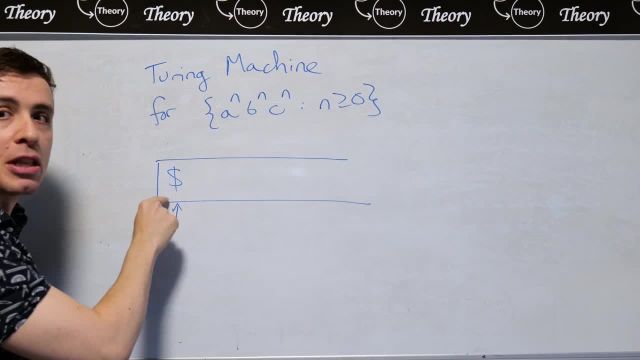 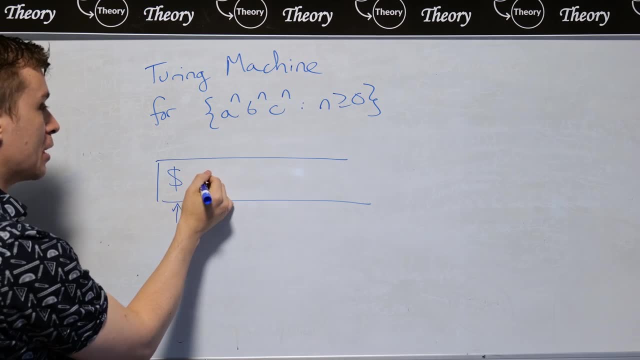 moving across the tape. we need some way of saying, okay, here's the thing at the very beginning, And actually for this problem there is a way of ignoring that, but I'm not going to look at that here. So let's just say that we have, let's say, three A's, three B's and three C's. Oh, that's another. 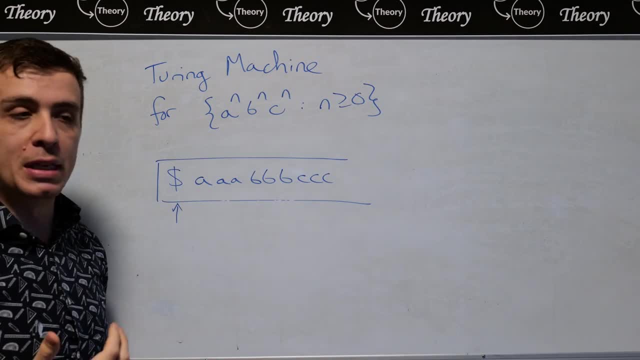 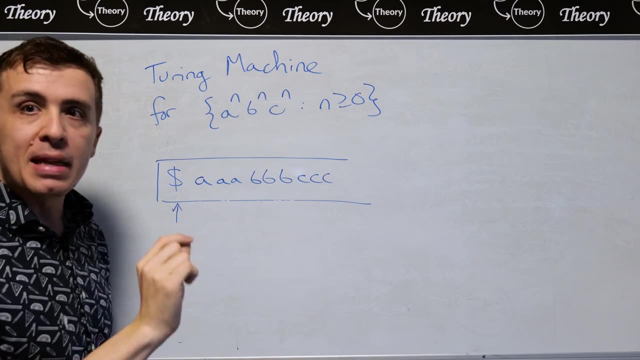 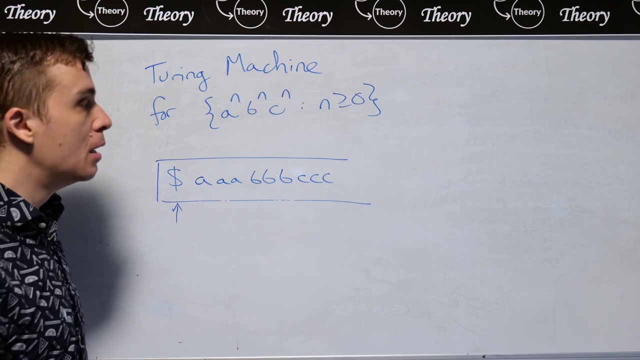 thing for Turing machines. The way to solve Turing machine problems is to think about solving the. assume that the input presented on the tape is correct and only make transitions for the correct things. So if you see something that is not valid at all, don't make a transition for it. 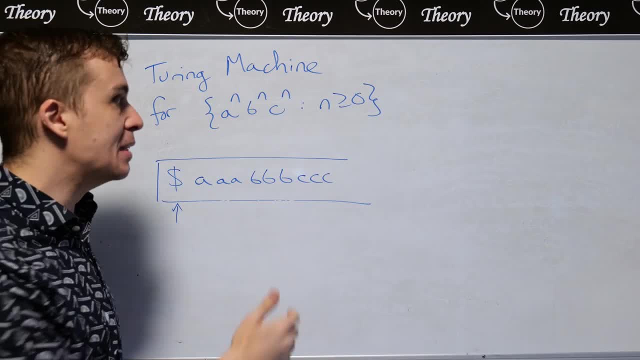 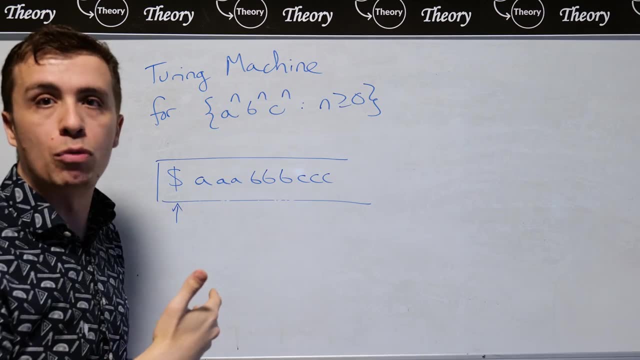 because if you leave out a transition, then that means that essentially you can just ignore it, because if the transition is not defined, the machine will reject immediately at that point if it needed to take that missing transition. So let's assume that we have a correct. 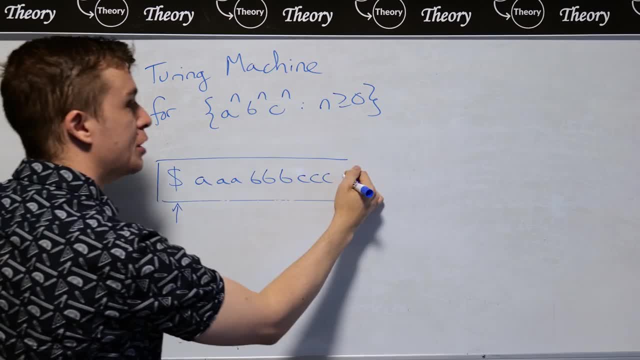 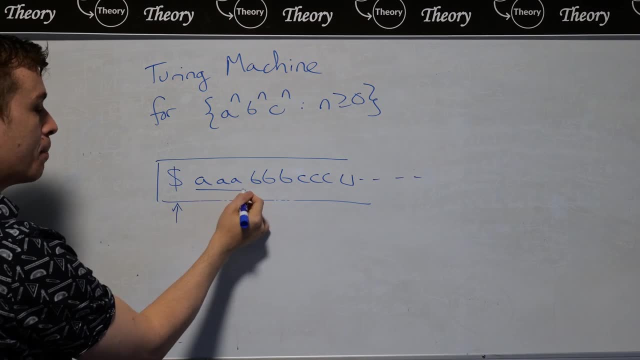 input right here, So it is in this language. And, of course, on a Turing machine there are blanks after the fact. So then, what can we do? Well, we got to ensure that the number of V's, the number of A's, is the same as the number of C's. sorry, the number of B's and the number of C's. 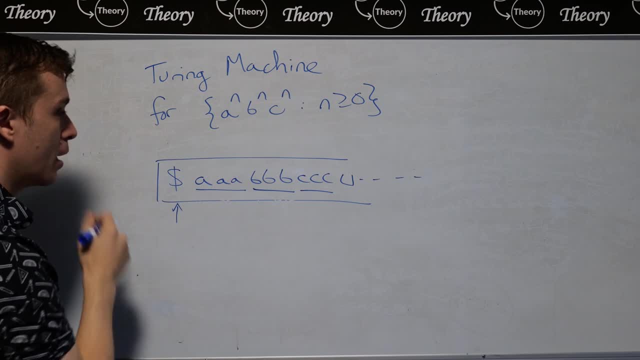 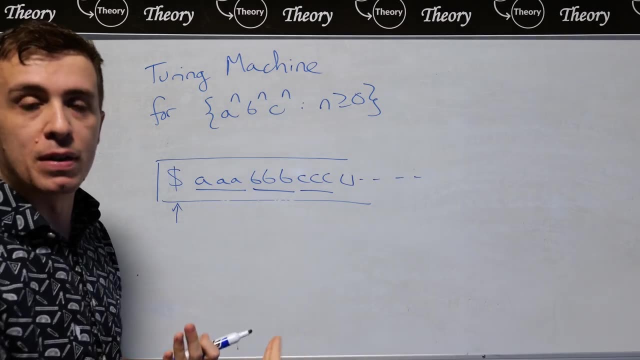 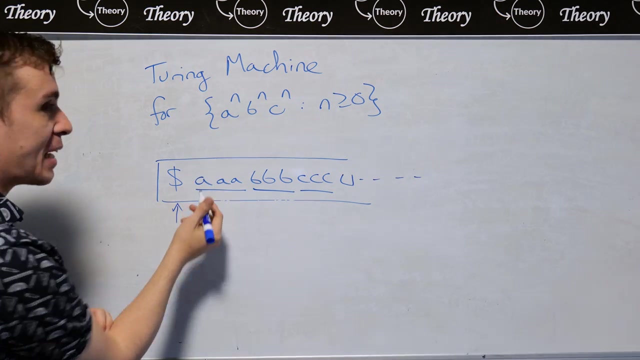 Exactly the same number, because that's what the language is saying. So there really is only one way to determine whether the count of something is equal to the count of another: one minus. maybe some small modification is to change some of these characters to other characters. So let's. 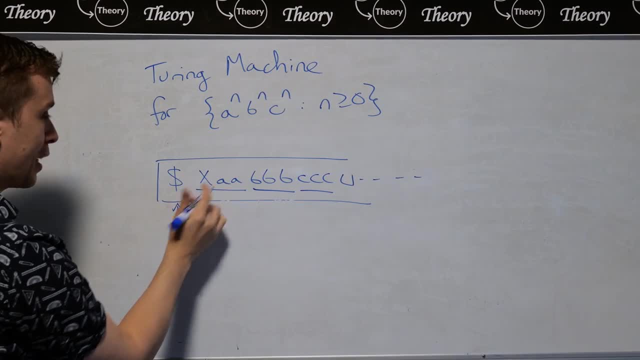 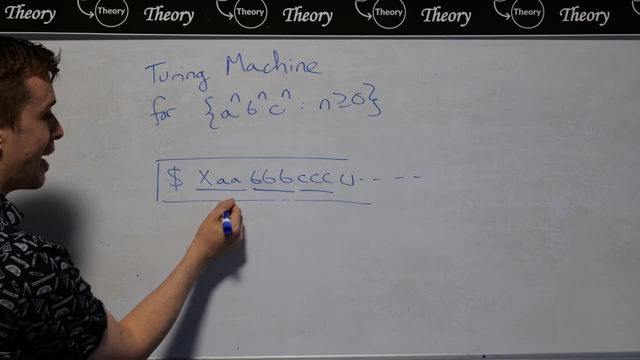 just say I change this first A into an X. So I move the tape head to this cell, I change it to an X, and let's say I moved right and so I'm not at that cell right now. So at this point we change. 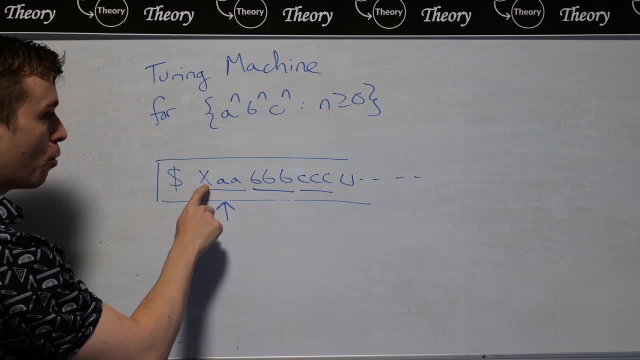 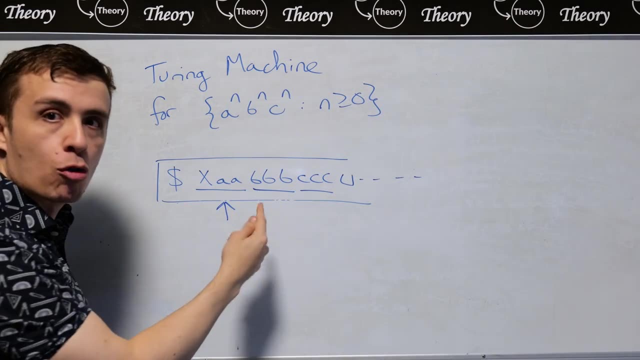 this A into an X, and then at that point we have marked one A, which means that if the counts are the same, we should be able to mark one B and then mark one C after the fact. So if we're able to, 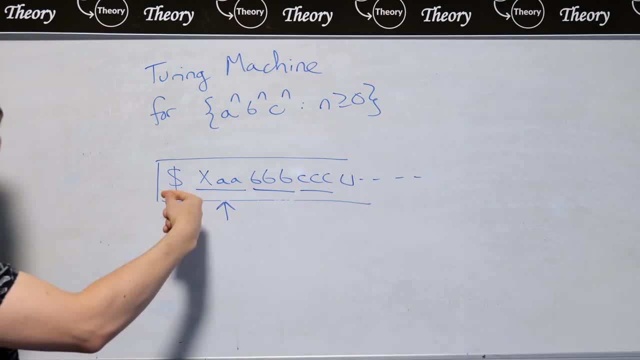 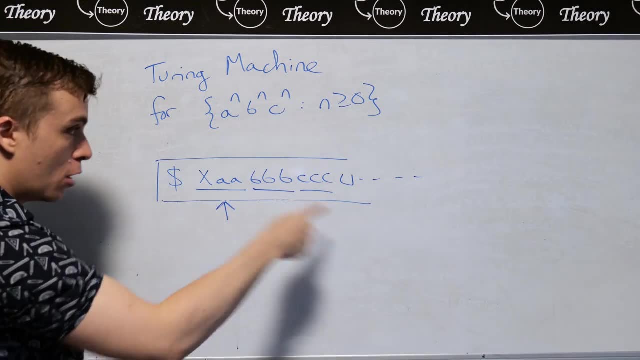 mark those, mark one of each. we go all the way back to the beginning and then mark one of each. So essentially, we're doing a zigzag pattern going across, over and over and over. There are many other ways you could have approached this, but this is the way that I'm going to approach it. 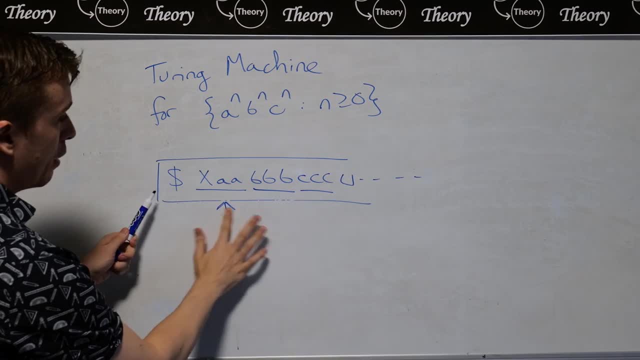 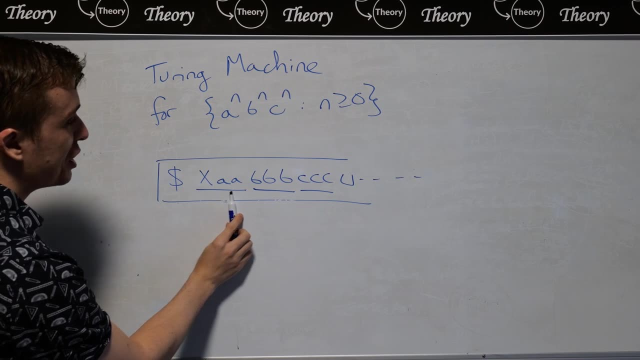 here. Okay, so let's carry this out though. So here we're at this position on the tape, so we're going to. we already marked one of the A's, so let's skip the rest of them, and then we haven't marked. we'll find the first unmarked B, which is right here. 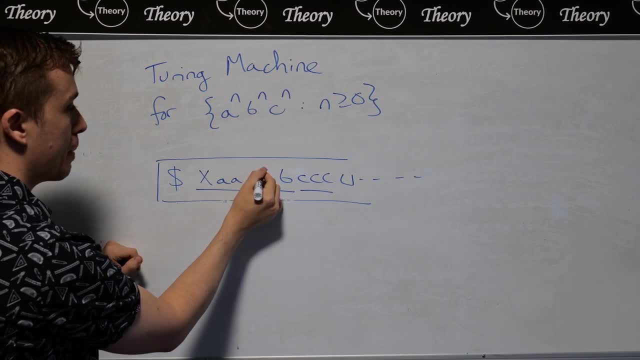 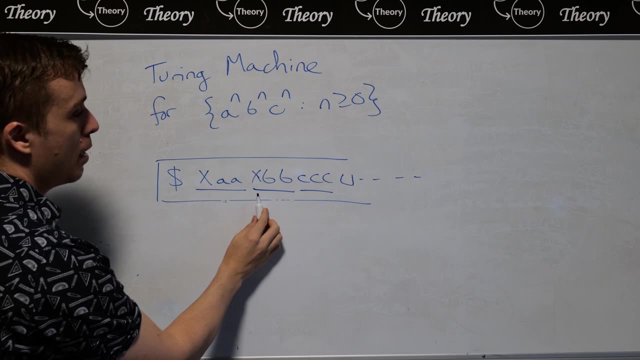 which I'm going to mark right here. Marking just means I'm going to change it to some character. Let's say I change it to an X. You could use a different character there you don't have to use the same one, but here I'm going to do the same character. So then I find the first unmarked C. 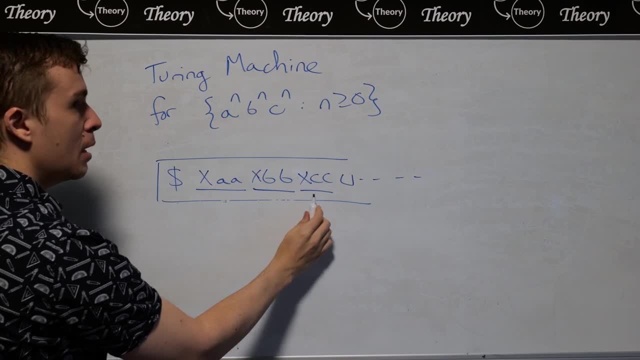 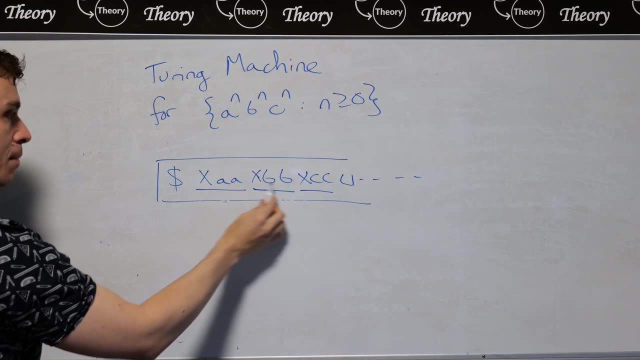 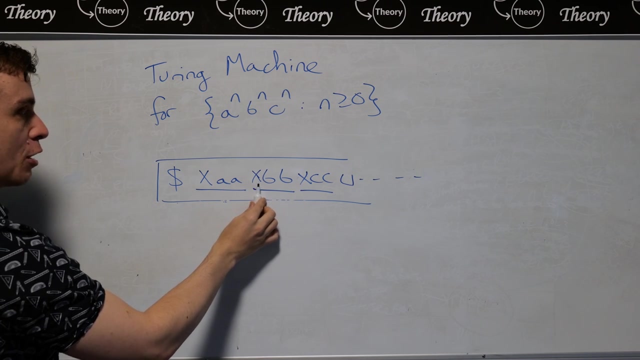 I mark it, which is, of course, means changing it to an X, and then, once I said okay, I am able to find a C. therefore, I'm going to scan back across all of the X's that might be over here, across all the B's that might be right here, across any X's that. 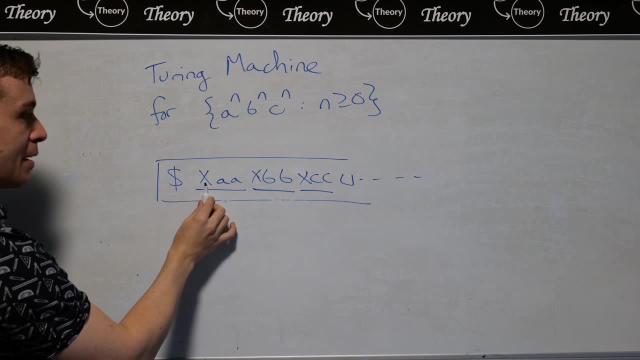 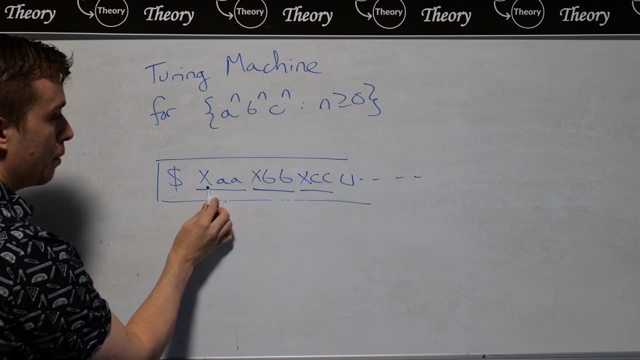 are right here, across any A's that are right here, and then I stop, let's say, at this X, although we don't have to, and then what I'm going to do is I'm going to move right one position. 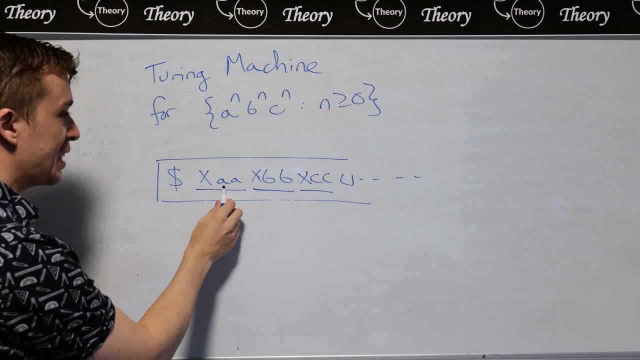 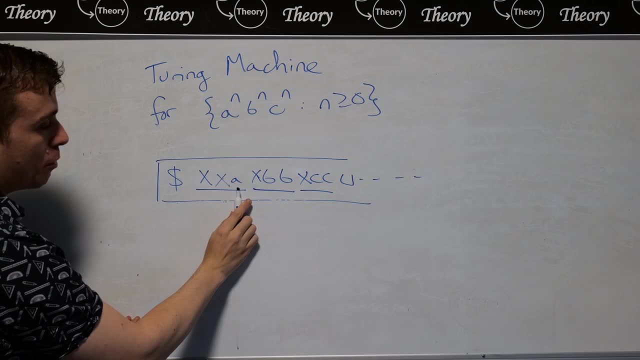 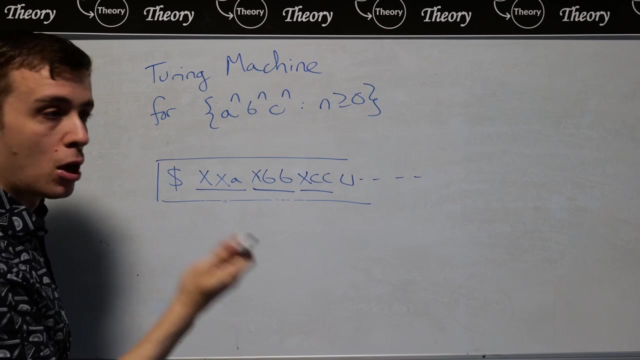 and then start the procedure again. So then I mark this A, so this one will become marked, so this is an X now. So then scan right past any other A's that there might be, scan across any of the X's that might be here, and then mark the first unmarked. 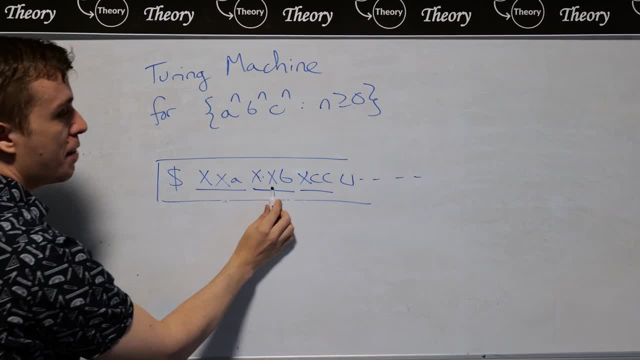 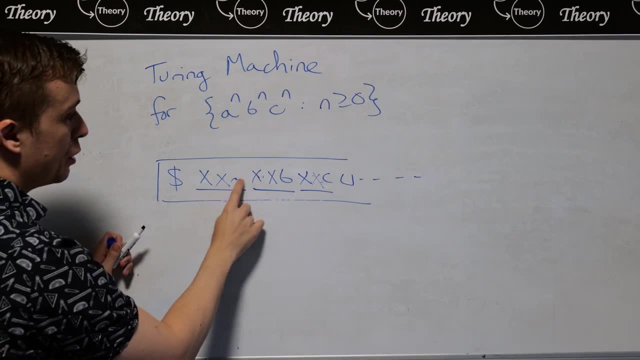 B, which is right here, So I mark that, and then go and find the first unmarked C, which is right here, and then we just keep zigzagging back and forth. So let's say we did this final iteration, so we've marked this last A right here. 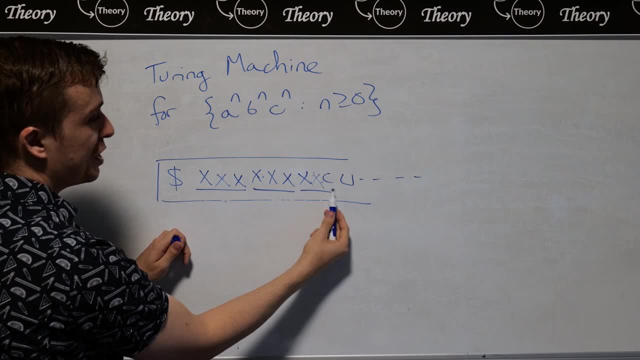 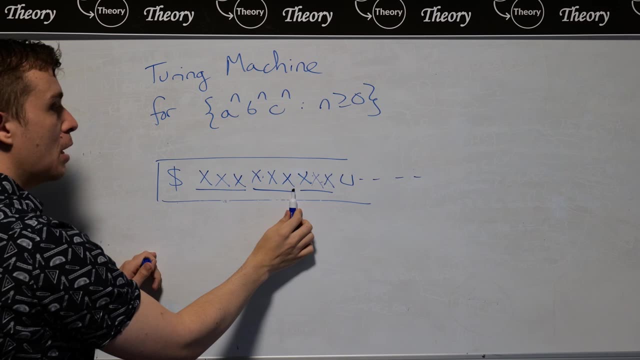 this last B right here, and now we're on the way to mark the C. So then, what we can do is say: so we mark the C right here. we're going to start scanning left. we don't find any C's, B's or A's, and let's say: we stop right here. 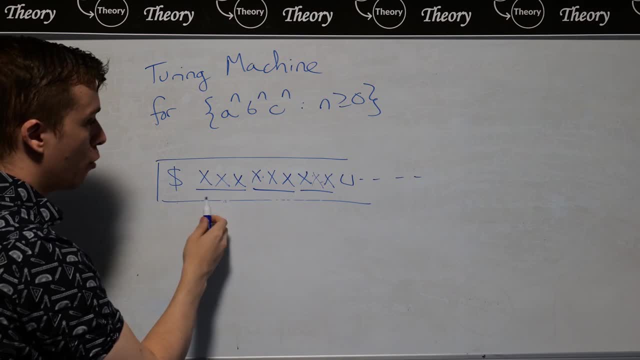 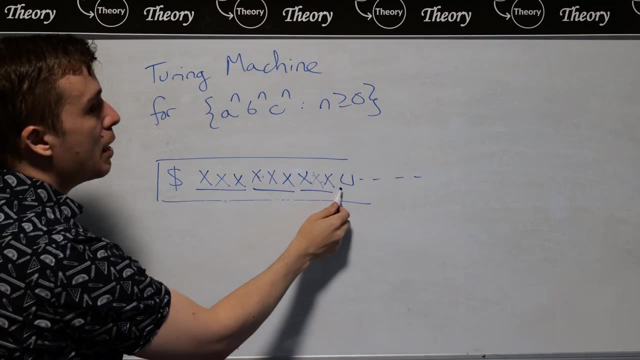 Then what we can then do to verify that we marked everything correctly is if we scan right over and over, and over and over past X's and never hit anything else, and we hit the blank symbol right here, we'll see that we've marked everything correctly. So then what we can do is we can 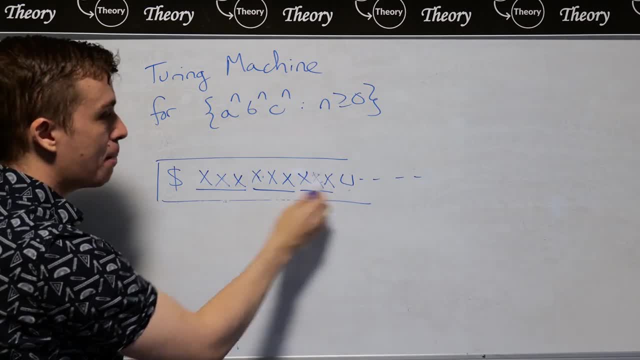 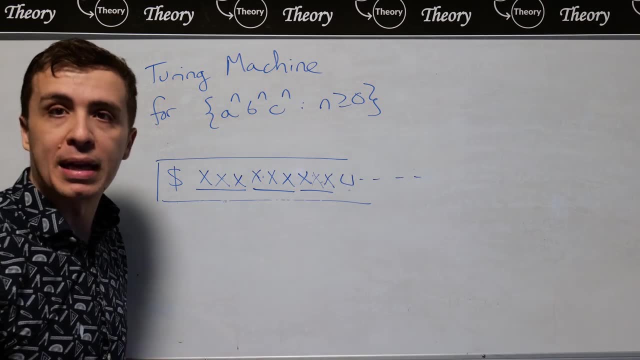 since we never wrote a blank anywhere else. if we hit a blank when scanning, right in this situation, that means that we have marked everything correctly and then, therefore, we can accept. So let's use this idea to solve this problem. So, actually, I'm going to leave the tape. 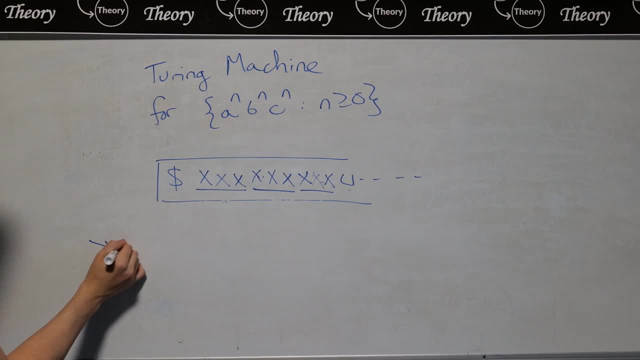 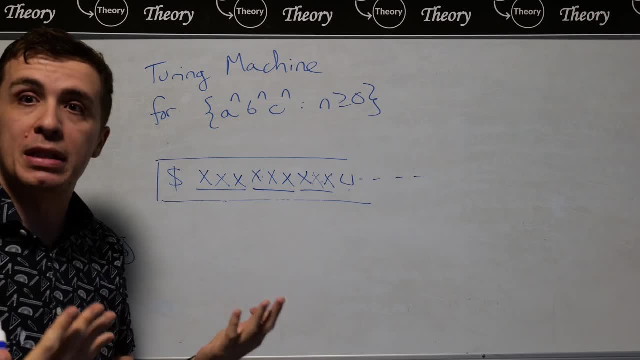 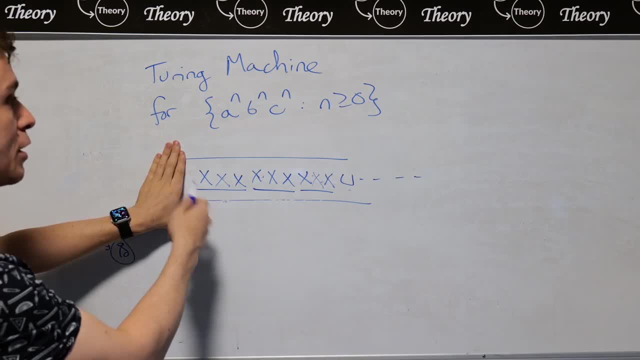 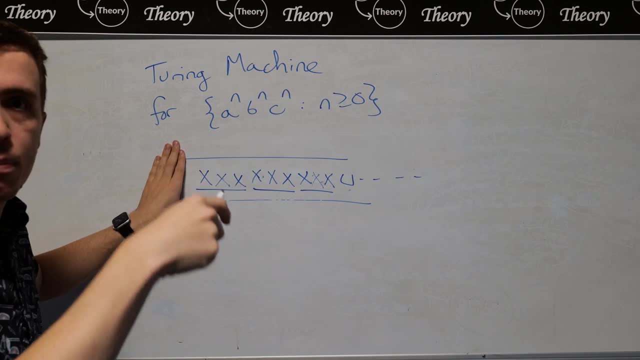 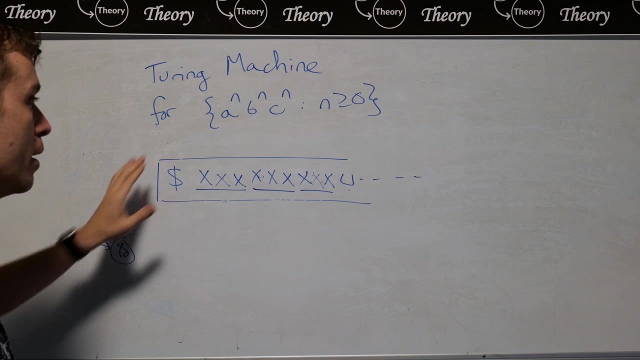 stand, and I shall mark it also by a capital letter: A. Ok, so we're gonna have a bad model here. We're gonna have a bad model here. So notice that I'm doing this in this, Okay, But actually notice how this is different. So I need to work on a different model right here in this. 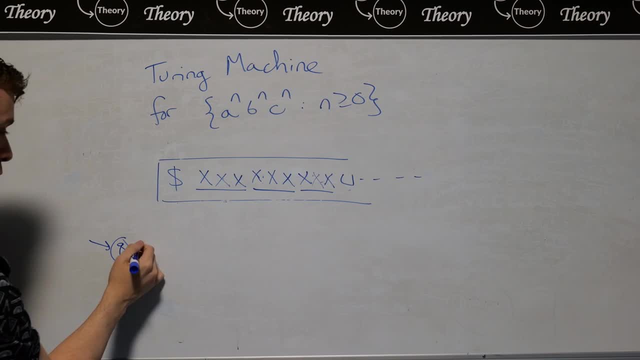 this dollar sign here, Although I could change it, but I'm not going to here, So I'm going to look at the dollar sign and skip right past it. So now I'm going to be looking at the A's, So at this point I'm going to call this state loop Again. 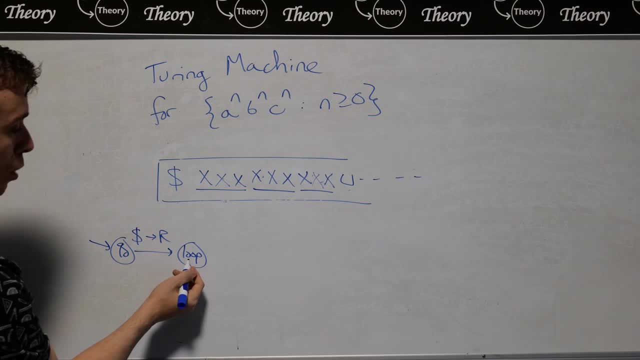 none of this is prepared. I'm doing this from scratch. But I'm calling this loop because at this point I'm going to be at the first unmarked A. So at this point, right here were at the first unmarked A. So here I want to actually mark one of 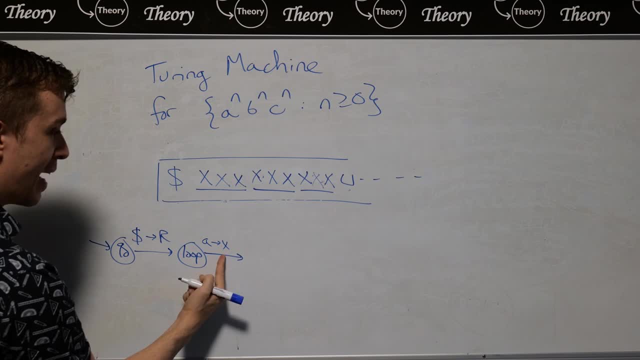 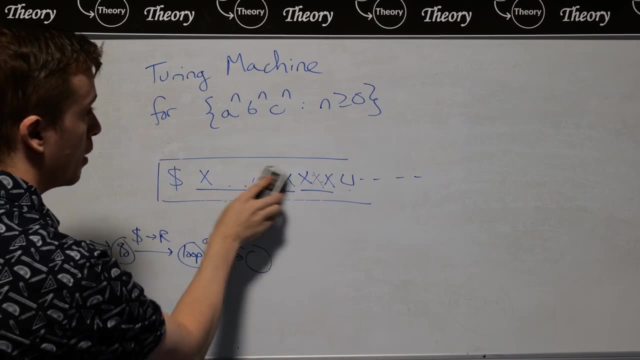 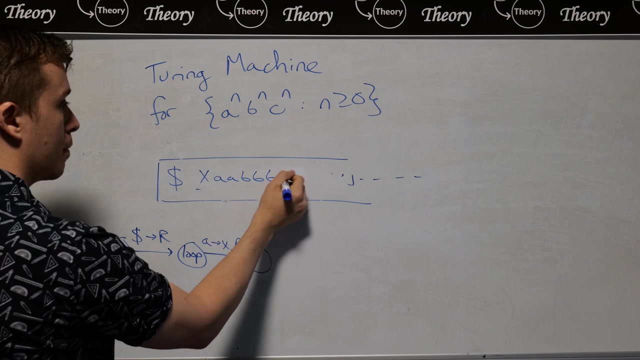 the A's. So here I'm going to have A, I'm going to mark it with an X right here and move right, And then let's see. so let's look at this situation right here. So at this situation, we we mark this thing. There could be some more A's and 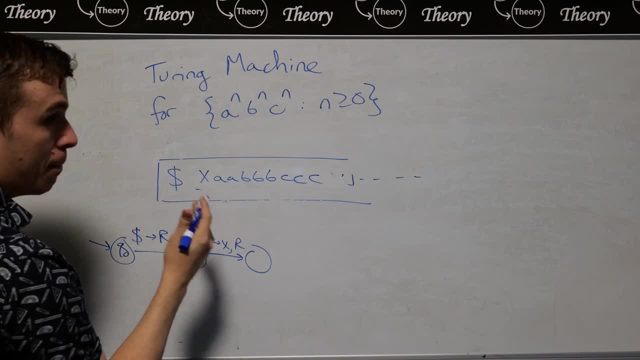 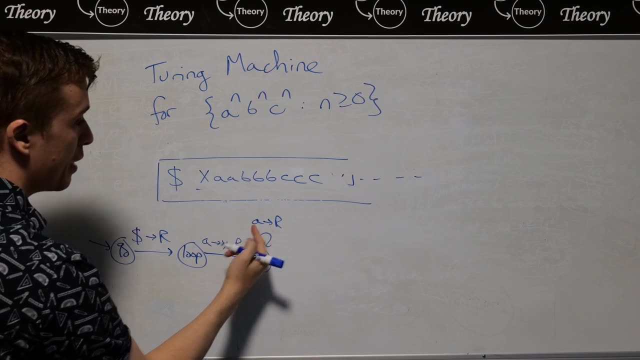 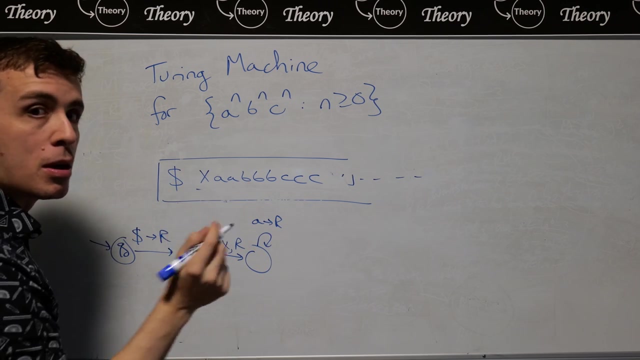 we don't and we have nothing else, mark at this situation potentially. So then here we could have some A's. So I'm just going to skip past any of the A's that there might be, Just skip past them. So then, at this point, what I want to do is I want to find the first unmarked B. 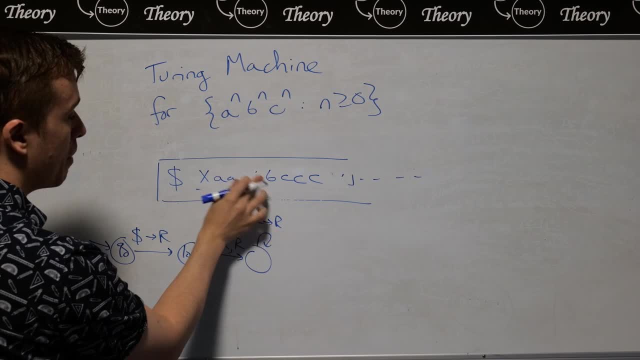 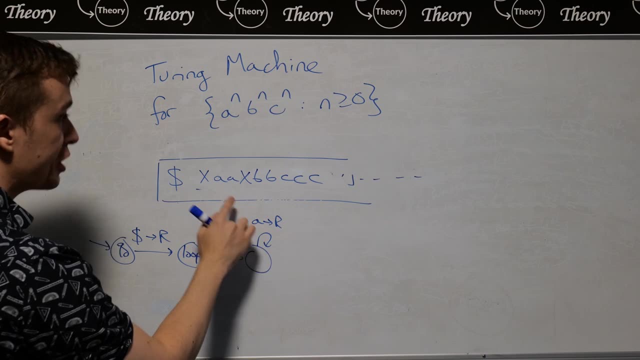 So at the very beginning, of course, there could be some X's. So, like something like this, There could be some X's right here. So, therefore, what I want to do is to skip past any of those that there might be also. 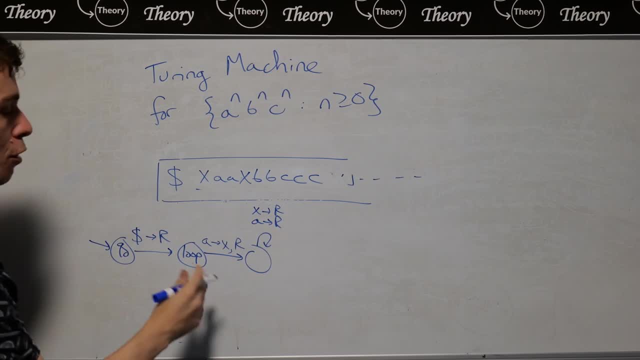 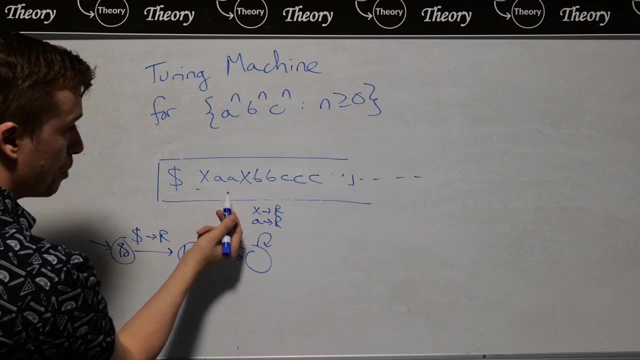 So I'm going to skip past any X's that are right here. There is a way to handle that. So you don't have both of these on the same self loop, but I'm going to have them both here. So at this point this state is going to skip past the A's, the X's. 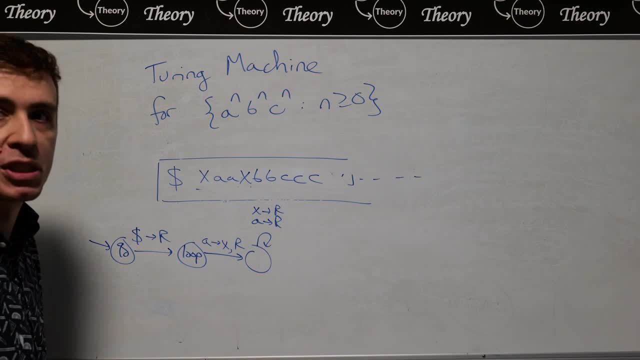 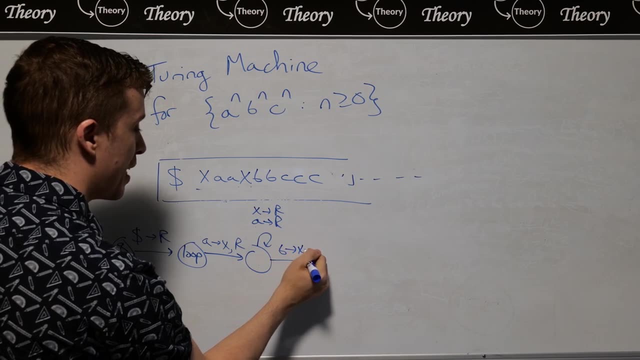 And so the first thing we should see- although we could, in principle, see other things- the first thing we should see is a B. So if we see a B at this point, I'm going to mark it with an X, exactly the same way we did right here. 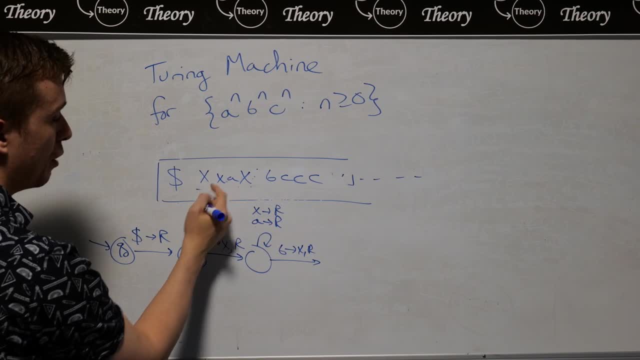 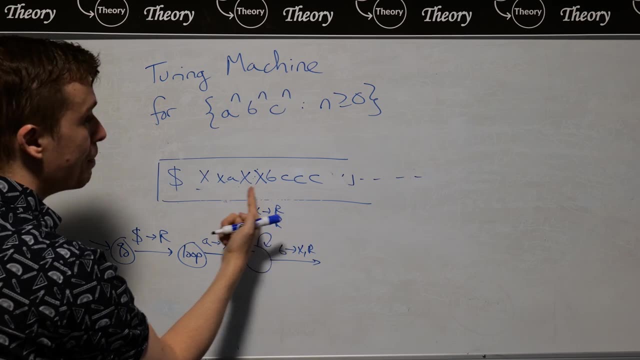 So this thing, in order for this to make sense there, So we mark this thing as a B, sorry, as an X right now, And so therefore, we have the same situation with B's and C's that we had with A's and B's before. 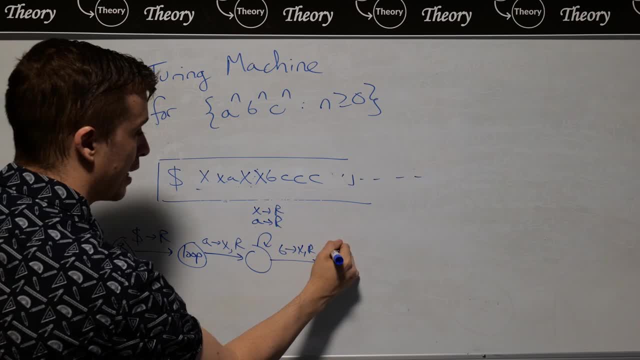 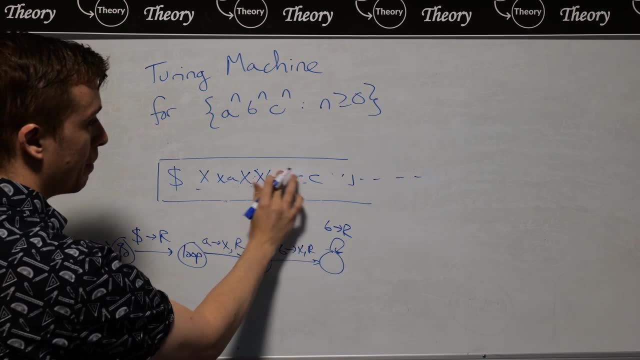 So at this point there could be some more B's left that I just need to skip past. So just skip past all of the B's that there might be, And then there could be some. in this case, there will be one. 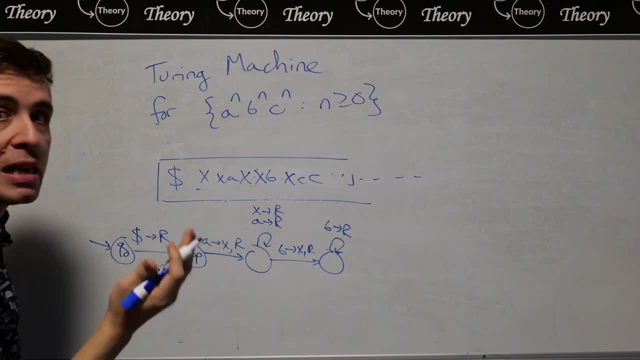 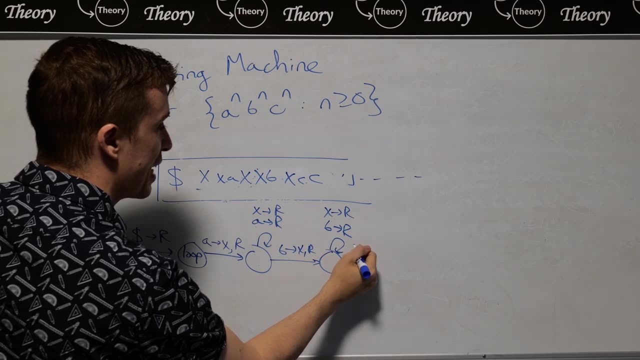 There could be some X's right here that denote the things that were marked in the in the C region, So let's skip past those, And then what I should see is a C. So then, if I'm right here, that means I'm going to mark it. 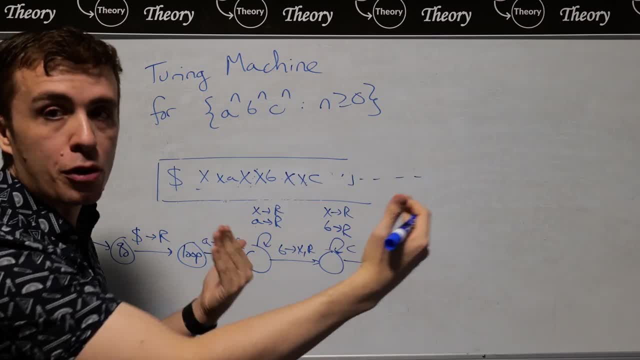 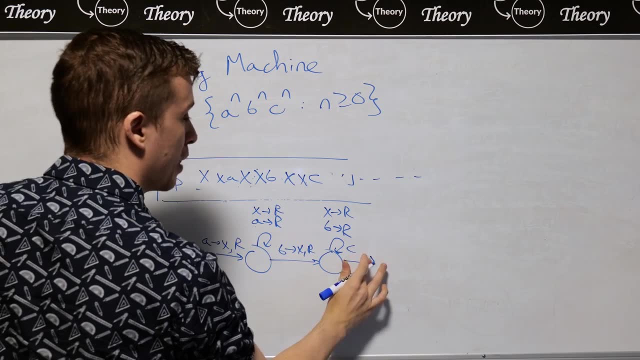 Then, at this point, I don't need to search any further, because I might need to do another iteration or I don't need to search for the right element. So, therefore, what I'm going to do is I'm going to go left. 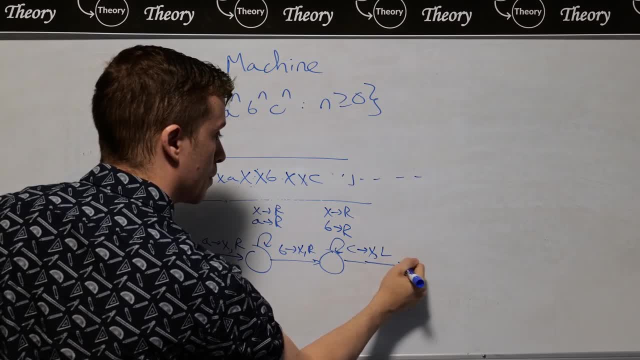 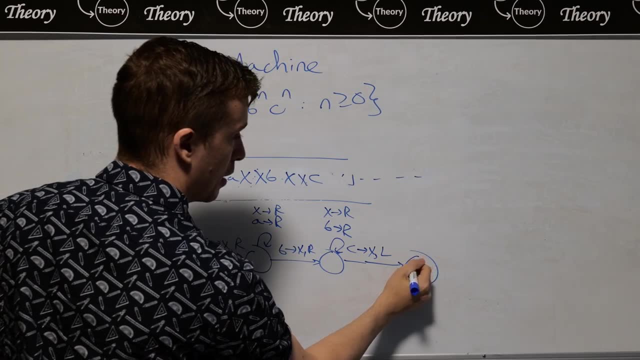 So I'm going to mark this thing with an X and move left. So then at this point we need to go all the way back over here. So I'm going to make a state called go back. Beatles will love that one. 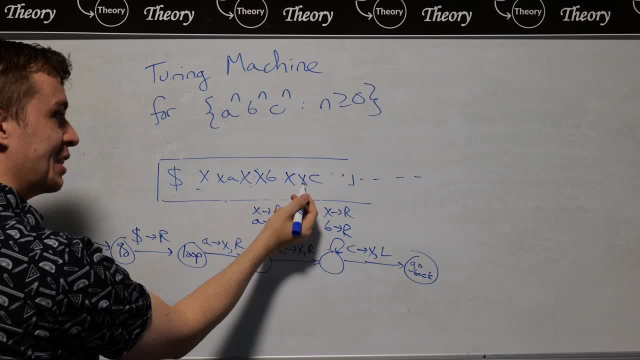 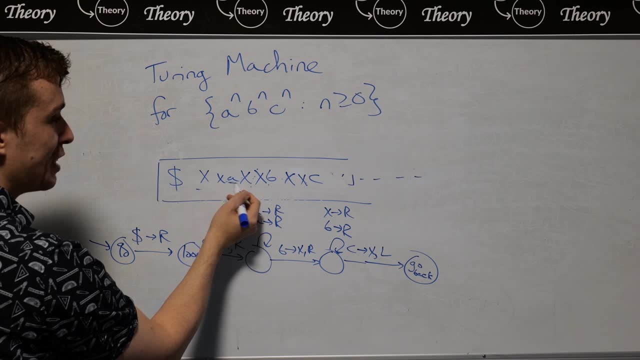 So go back. So the things that I can see along the way are X's. I can't see C's, B's and A's, So I need to skip past any A's that there might be, any X's that there might be. 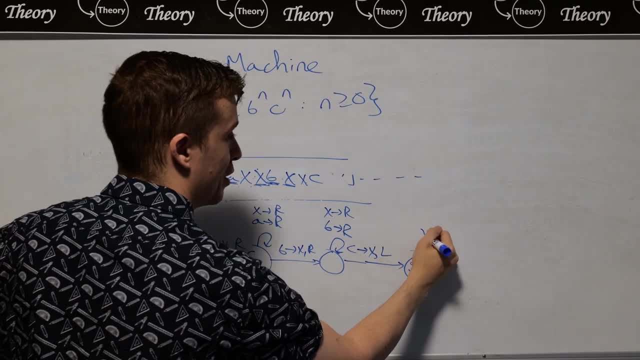 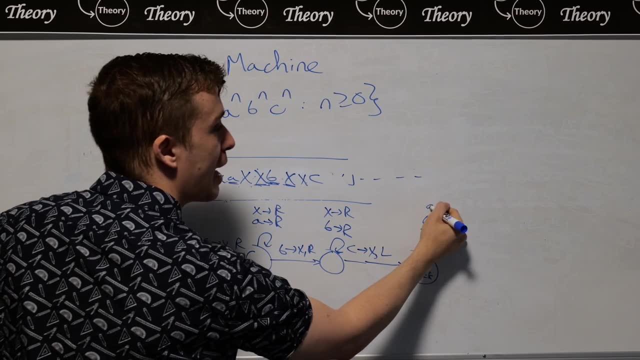 and any B's that there might be. That's a funny sentence. So I'm going to have an X, I'm going to skip past it, going left. Any B's, I skip past it, going left. And any A's, I skip past them, going left. 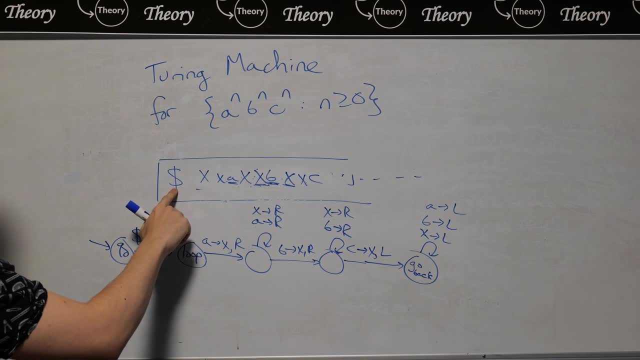 And then, if I see the dollar sign I'm going to, I need to go past that dollar sign to find the first unmarked A, because that's what this state is expecting, Although there's another way you could have done it. So here, what I'm going to do is go to a state right here. 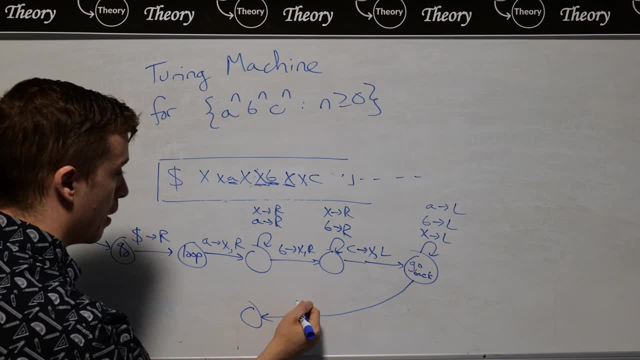 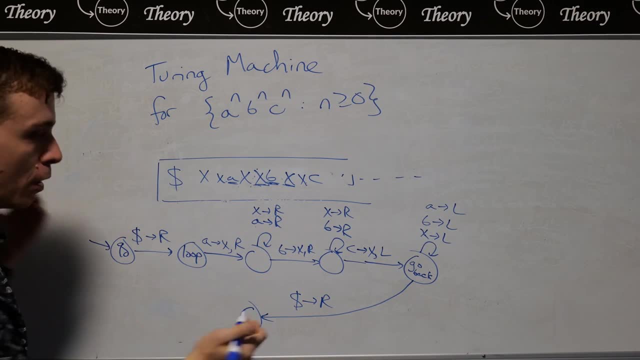 So this transition is going to have dollar sign goes to right. I don't want to change that because that's my stopping point, if you will. So I'm going to go past the dollar sign. So I'm right here in this state. 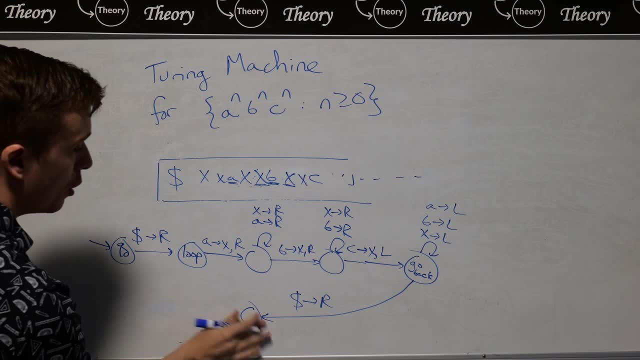 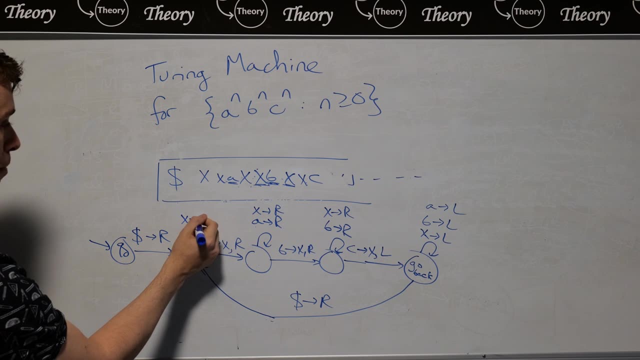 So then, what I'm going to do is Actually: no, I'm going to do this, So I'm going to go directly to that state and then skip past any X's that there might be in this state. So here, this R is going to go to the very first A that there was originally. 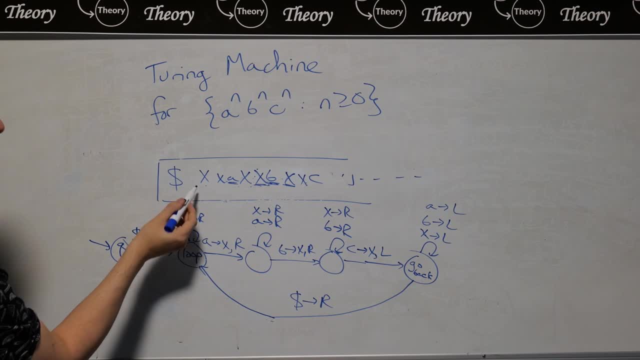 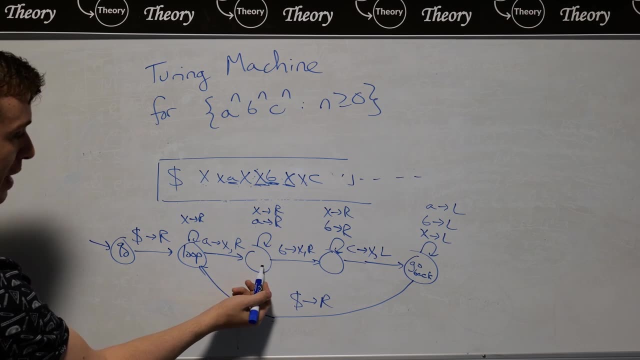 but it could have been X after some iterations around. So therefore it's going to be, let's say, an X. So therefore I'm going to skip past them, and then eventually I might hit an A. Well, let's just say we don't hit an A. 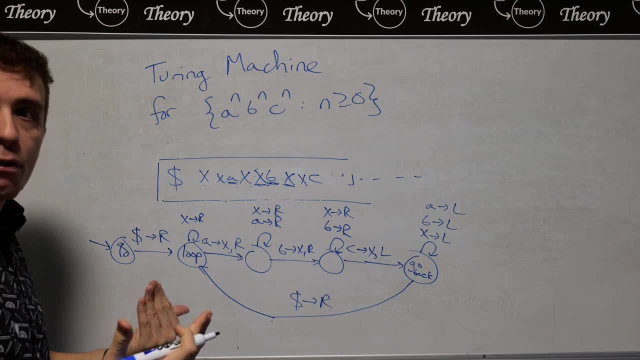 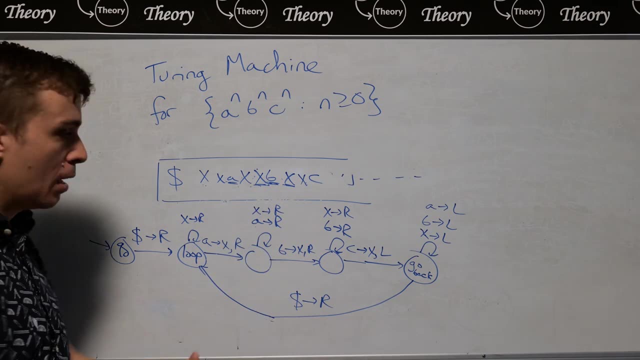 If we don't hit an A, the only thing that we really care about for accepting is if we hit the blank at the very end. Note that if we hit a, B, I don't care, because those transitions that are not written are going to go to the reject state. 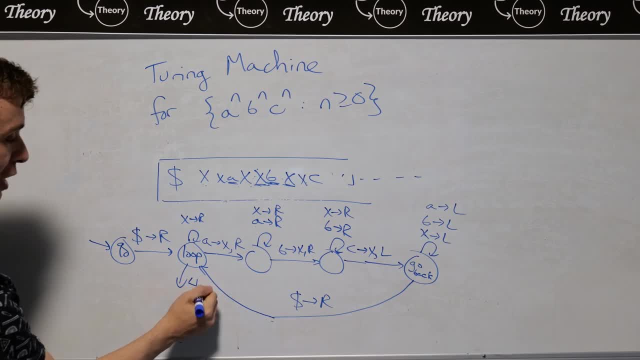 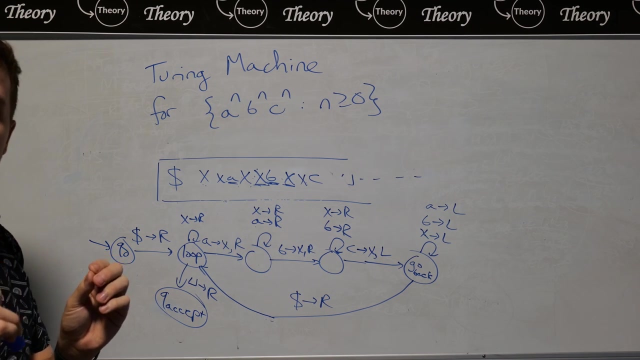 So what I'm going to do is, if I see a blank symbol, I'm just going to go right. There's no reason to go left here And then go to the accept state, And I don't need to do anything else. So the thing to note with Turing machines is: 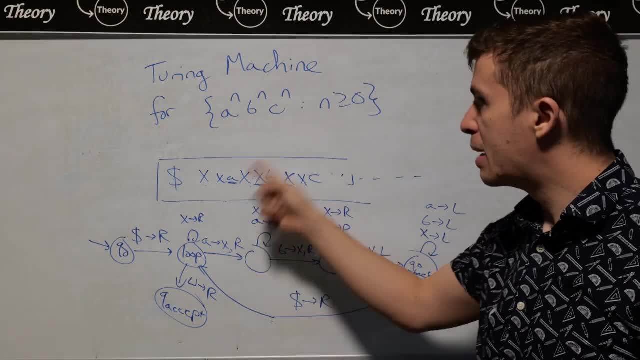 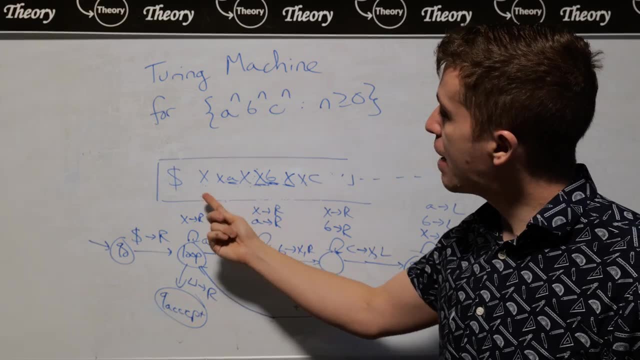 let's consider if we have the empty input. So if we have a non-empty input, it's pretty clear that this does the right thing, unless I made a small mistake. But let's consider the empty input. Well, if we have empty input in this model, 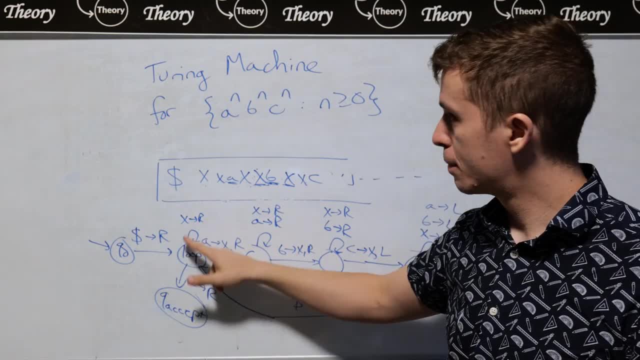 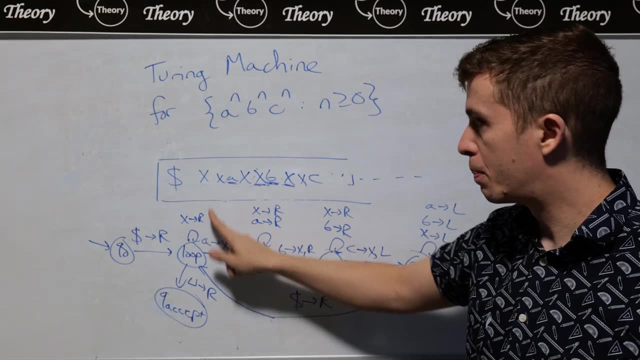 we have a dollar sign right here and a blank symbol right here. So let's consider what happens. So Q you see the dollar sign, we move right, we go to the first cell, which is a blank, and therefore we go down here. 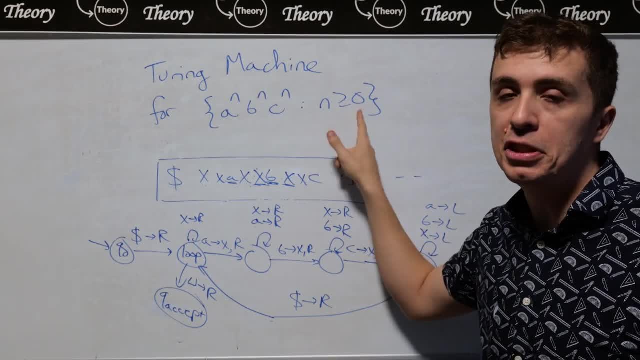 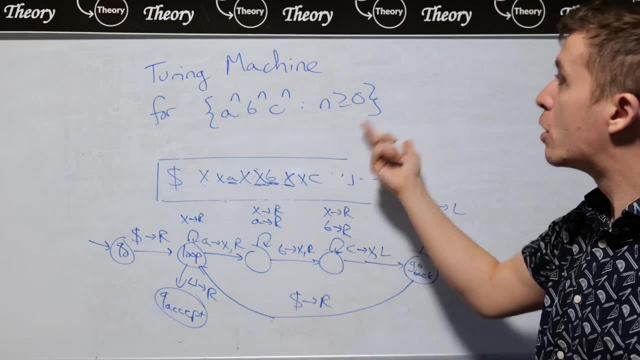 And we should accept it because n is at least 0 here. So if n is 0, that's the empty string, which is exactly what we want, And if we have n bigger than 0, so that means that there is some A. 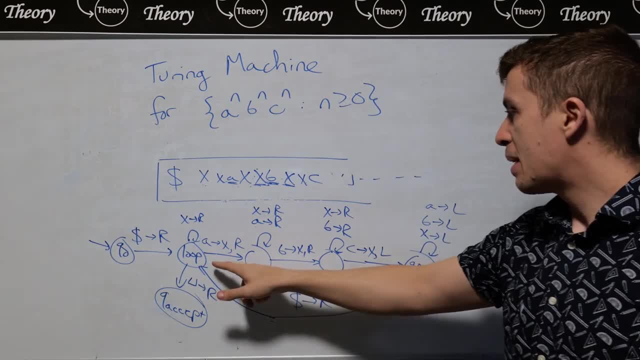 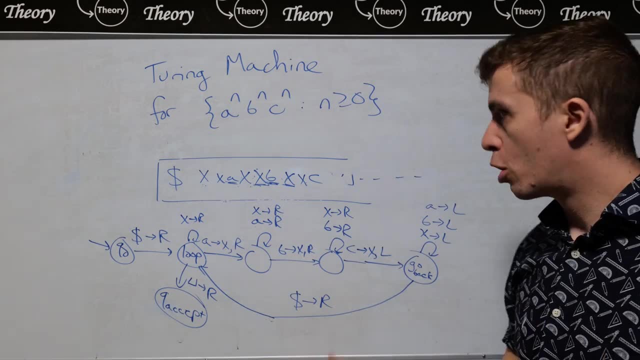 some A, B, some C, then that means that we will take this transition and then we'll go around the loop as we were discussing earlier, And if the counts aren't correct, then at some point one of these is going to be the minimum. 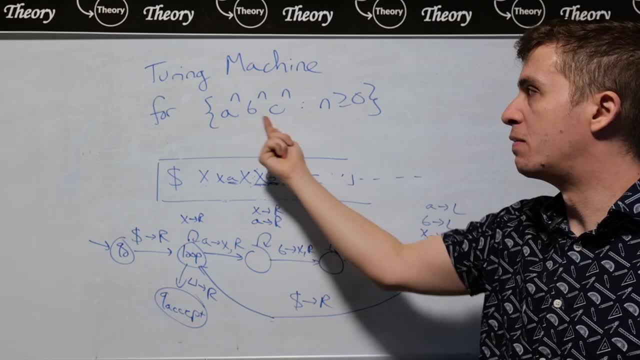 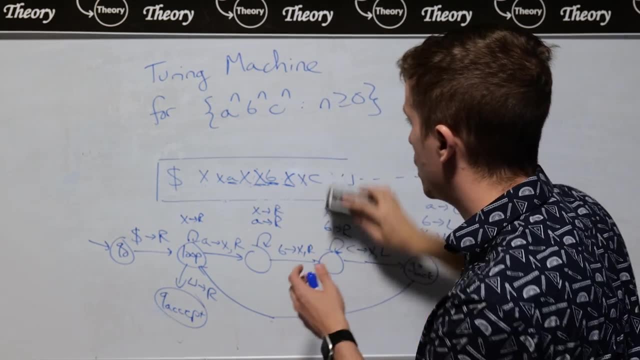 whichever one it is, Let's say that A is the smallest of the two, So which shouldn't be accepted. So if we have, let's do a short example. So if I have, let's say one A and two Bs and two Cs. 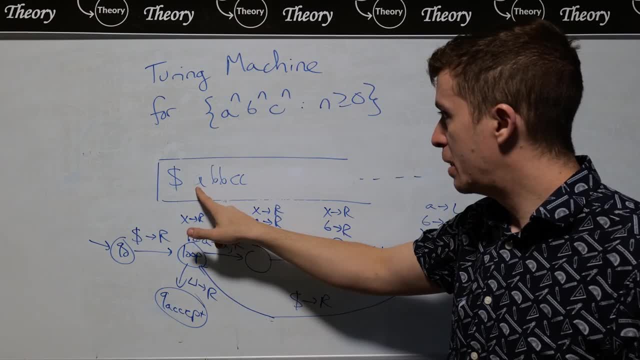 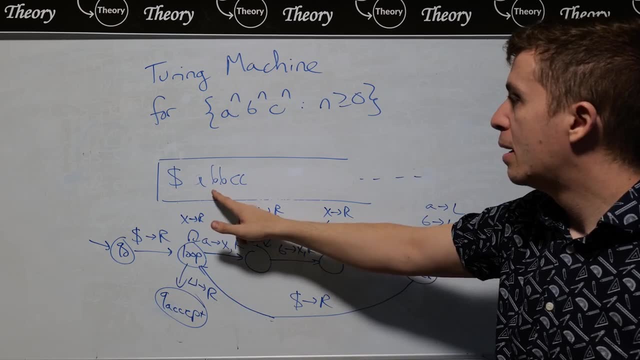 then that means that I'm going to mark this A, mark this B, mark this C. go back, then I'm going to hit the dollar sign. try to scan right, looking for either an A, an X or a blank symbol. 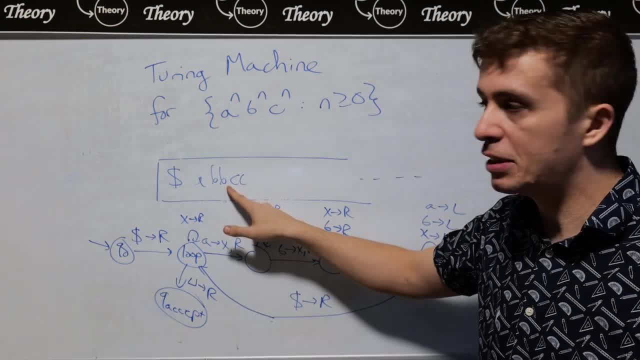 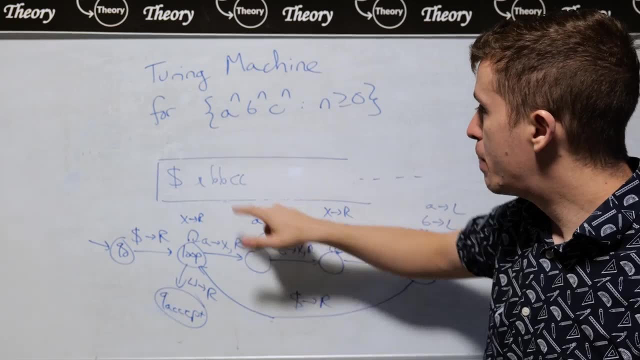 Well, the X is, I just skip over. I can't find an A because there isn't any, and I don't hit the blank before I hit something else, so the machine will reject. If we have a fewer number of Bs, then at some point. 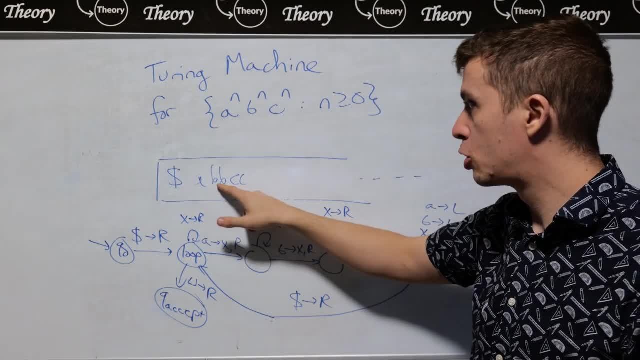 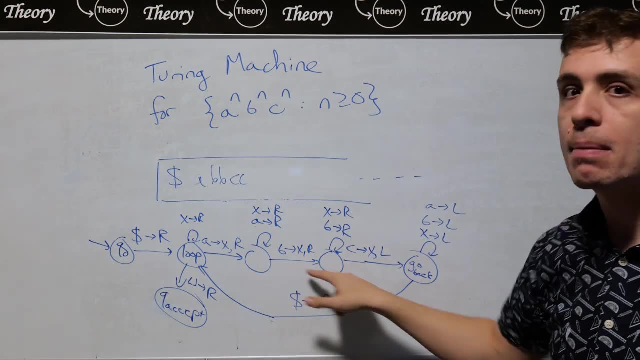 we're going to exhaust this, that that whole section, and there's going to be some As left, which means that I'm going to mark one of the As and not be able to mark a- B, so we're going to get stuck in this transition. 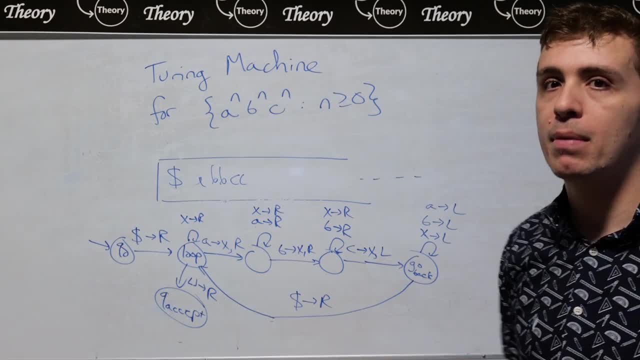 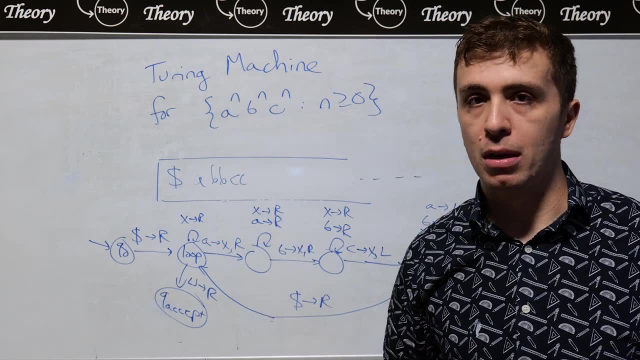 or we can be stuck in this one if the Cs are the minimum. So therefore this machine, unless I made a very tiny mistake, is a Turing machine for this particular language. So hopefully this gives you some insight into how I solve Turing machine problems.